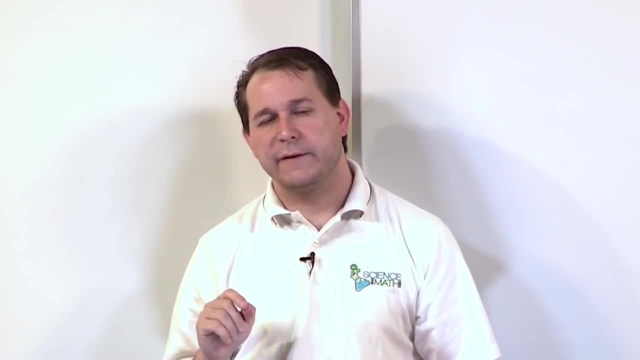 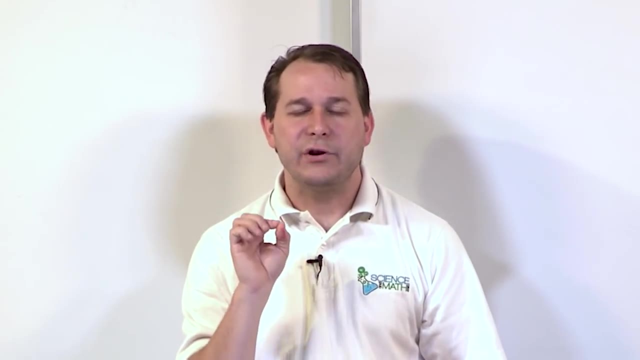 down and it's very important. That is that and I want you to remember this. when you have a fraction, remember there's a numerator on the top and the denominator on the bottom- whenever you have a fraction, you can multiply that fraction by anything you want, any number. 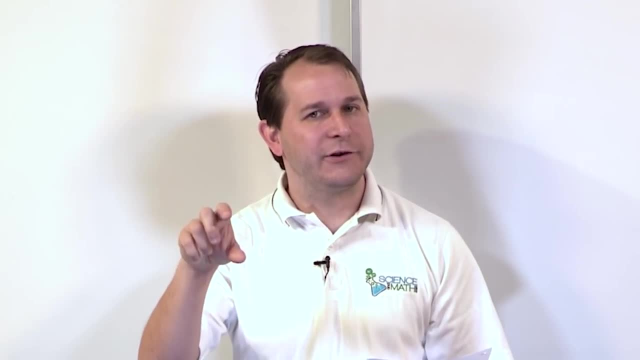 you want, As long as you multiply the top of the fraction by the bottom. you can multiply the fraction by anything you want, any number you want, as long as you multiply the top of the fraction and the bottom of the fraction by the same number. So if you want to multiply, the top of the fraction by 4, that's okay as long as you multiply the bottom of the fraction by 4. also, You can multiply the top of the fraction by 16 if you want to, but the only thing is you have to make sure and multiply the bottom of that fraction by 16. 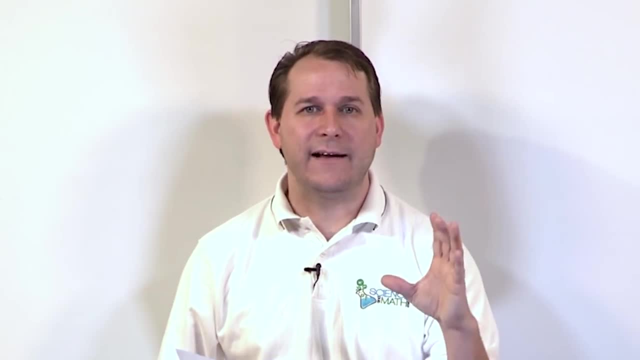 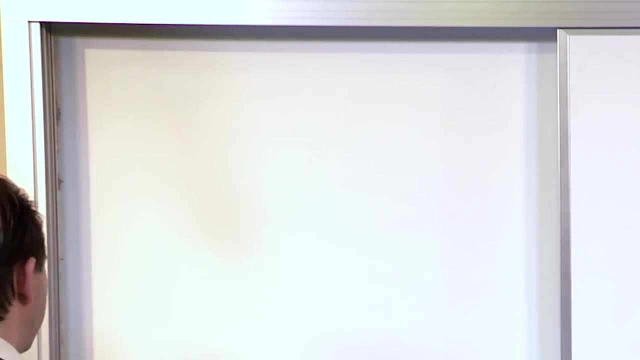 as well. So when you do that, you keep the fraction in balance, and that's how you make them and see that they're equivalent. So let's draw a picture of the most famous fraction of them all. Here's our pie, and 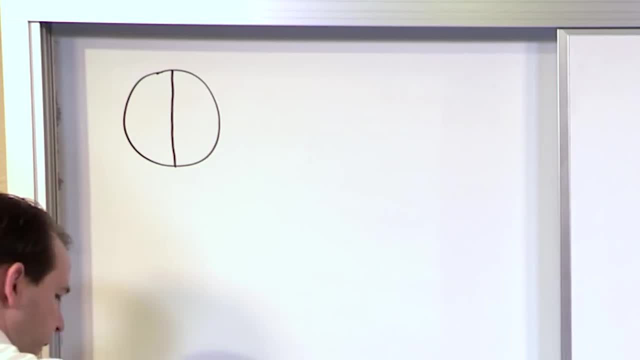 here. we've cut it exactly into two pieces, So let me go ahead and shade this guy. If this is the amount of pie that we actually have, what fraction do you think we have? Well, we have two pieces in total, and I only have one of these two pieces, so this is one. 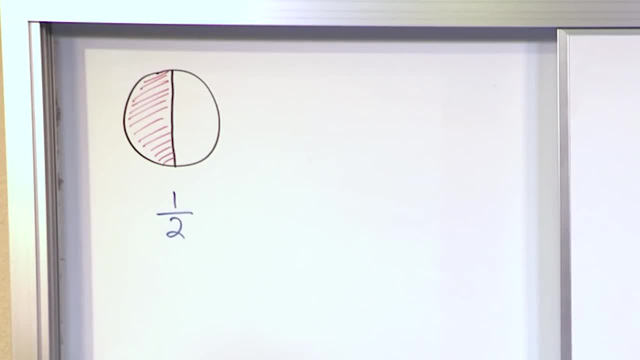 half. This is the most famous fraction of all. right, Half a piece of pie, half a piece of pizza, half a pie, half of a peanut butter and jelly sandwich or whatever. Alright, so let me show you something. What I can do is I can put an equal sign here and I can take. 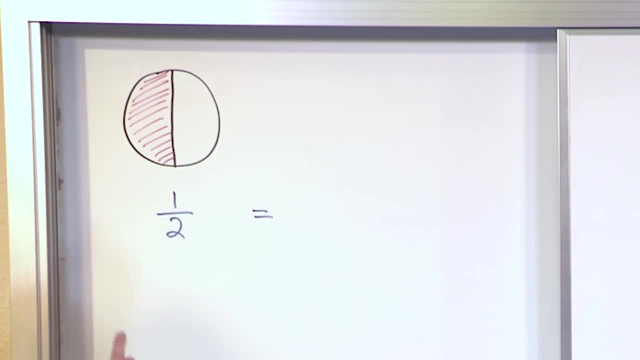 I told you, I can take the top and bottom of this fraction and I can multiply it by anything I want, as long as I do it to the top and also to the bottom. So I can rewrite my one half and I'll just make a longer little fraction bar here and I can multiply the. 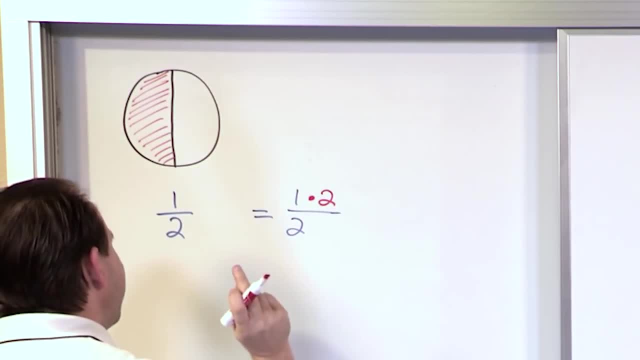 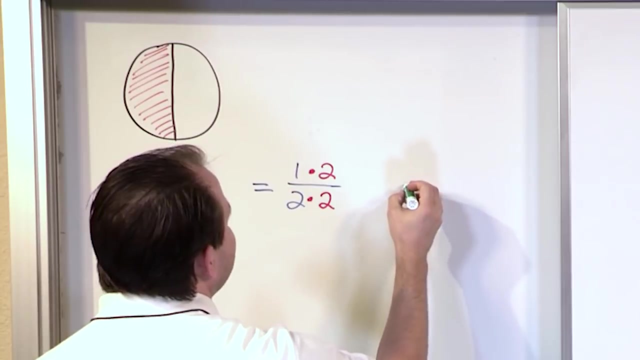 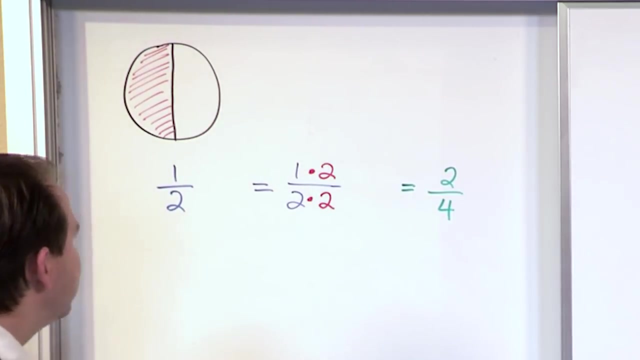 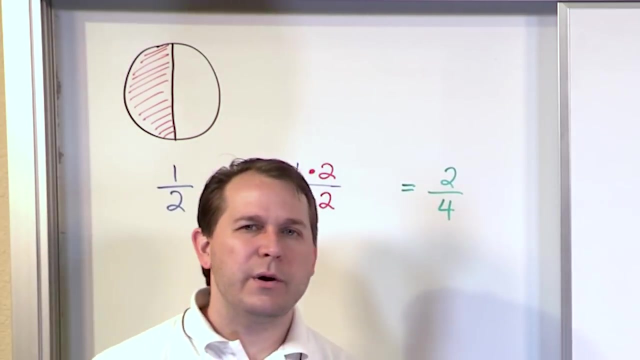 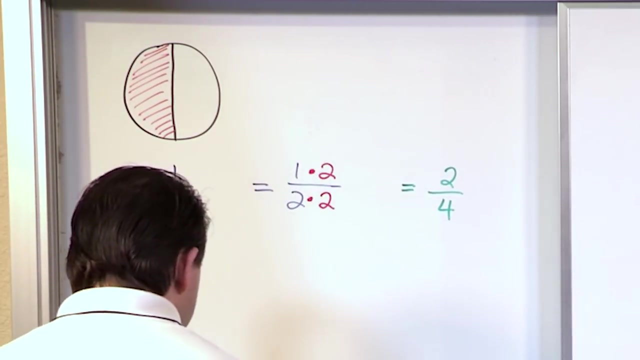 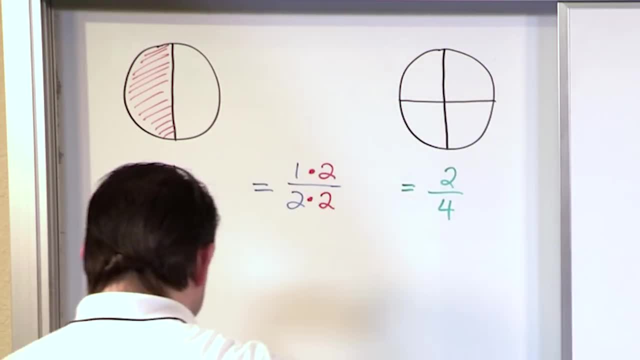 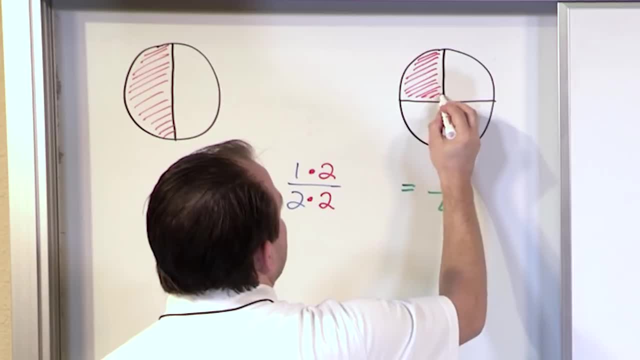 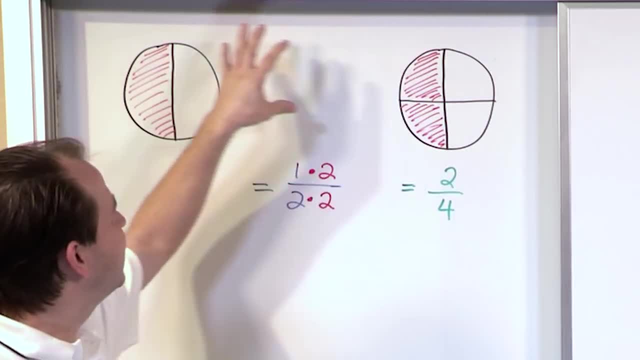 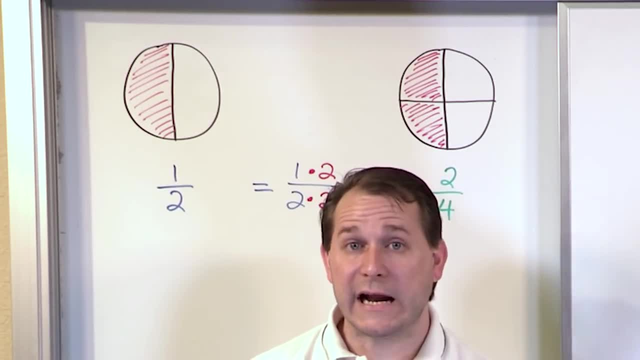 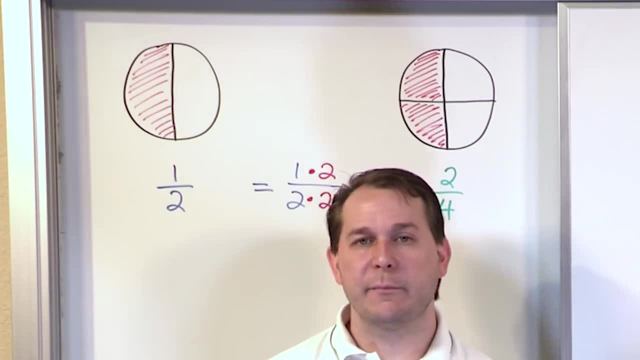 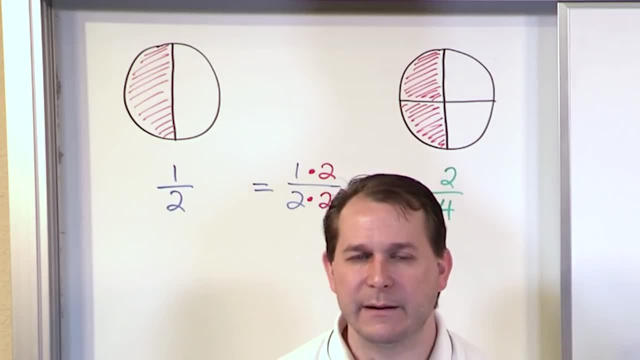 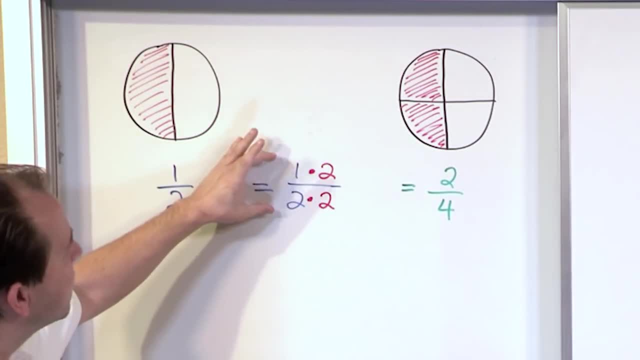 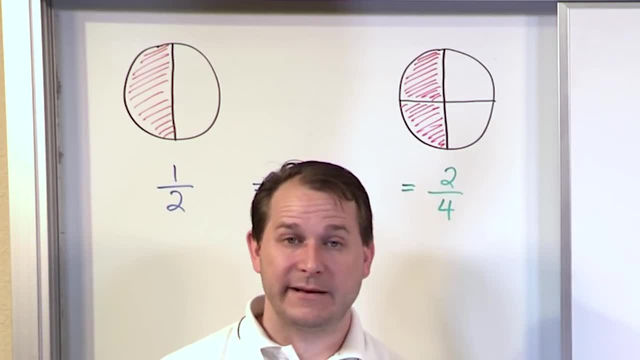 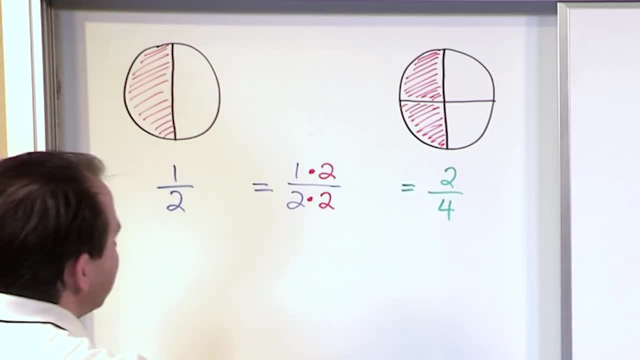 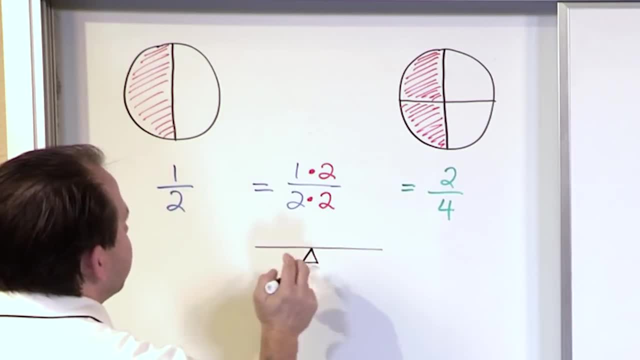 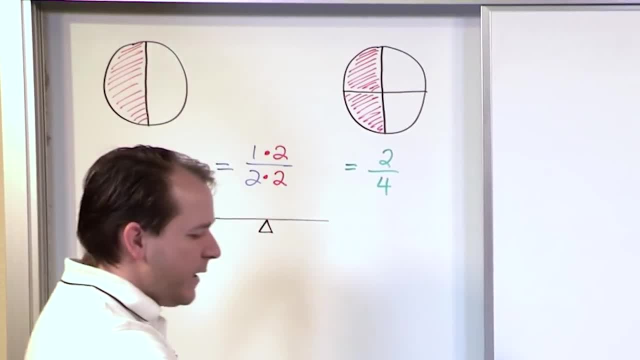 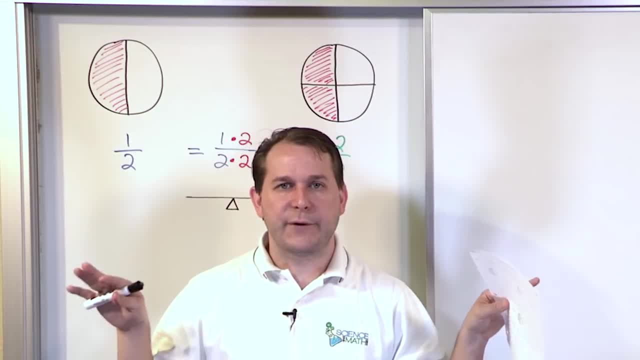 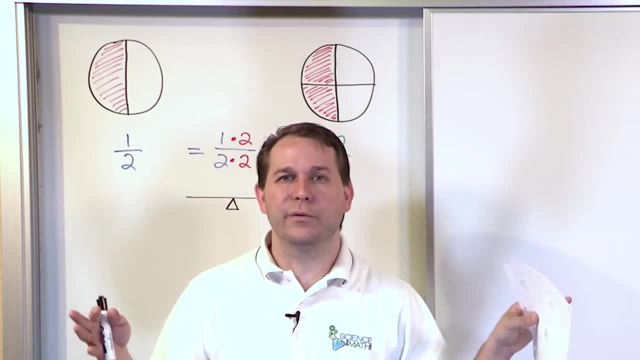 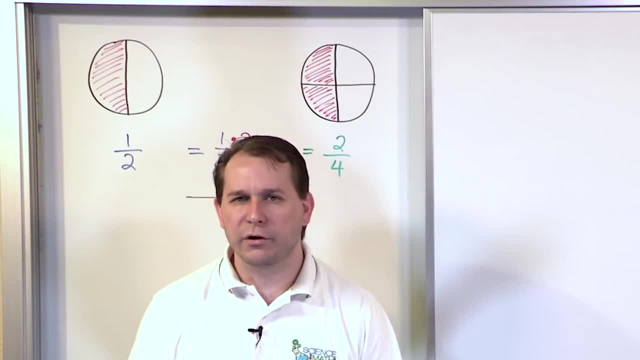 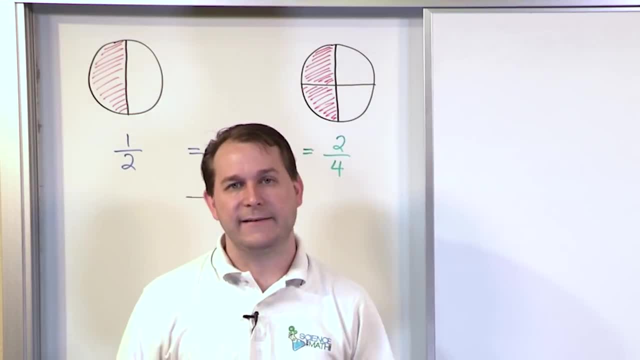 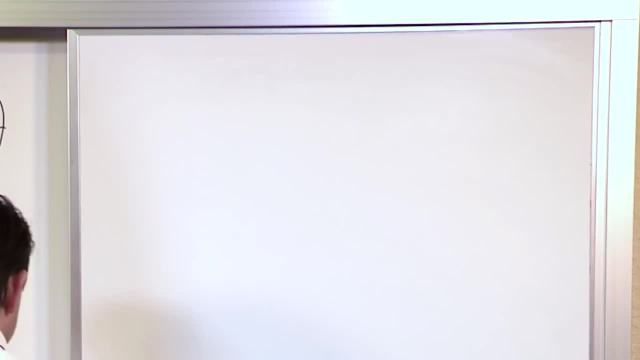 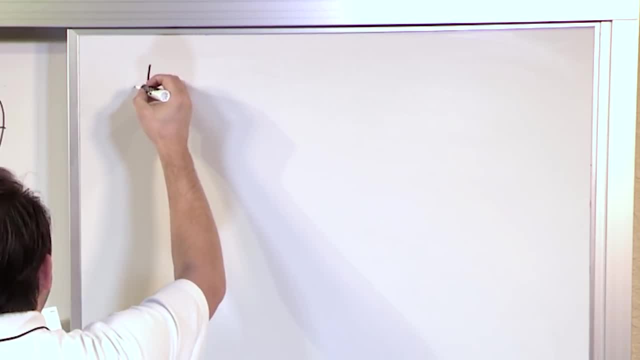 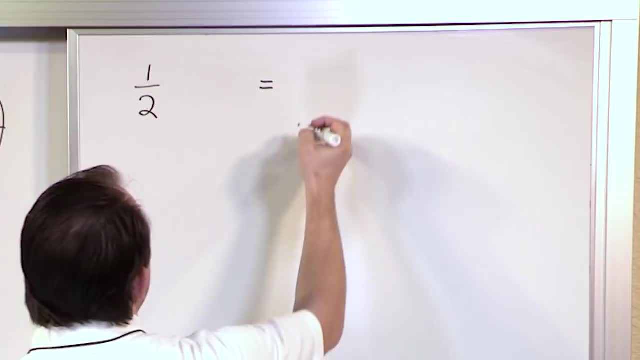 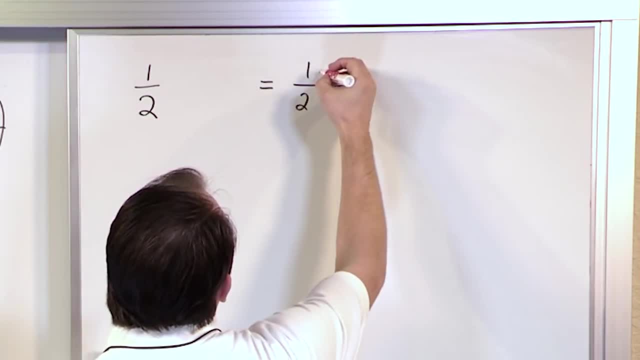 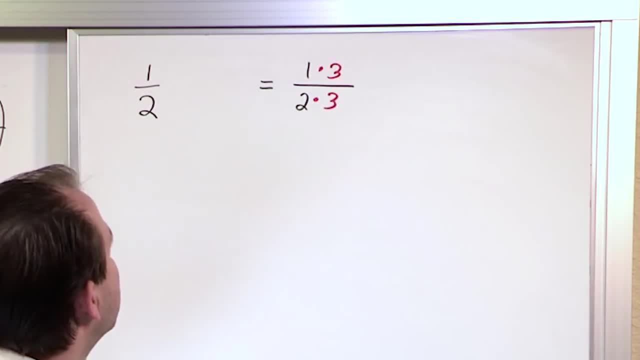 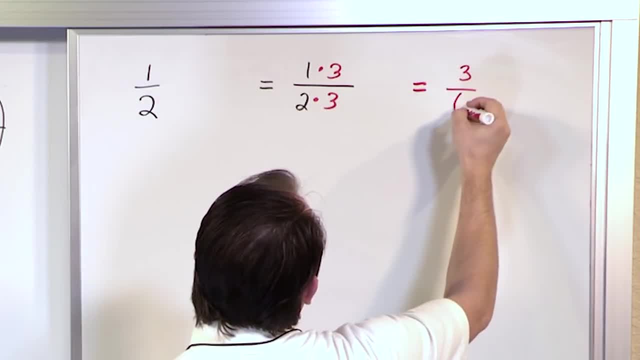 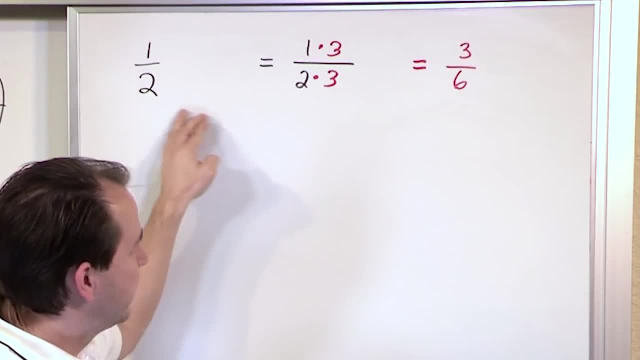 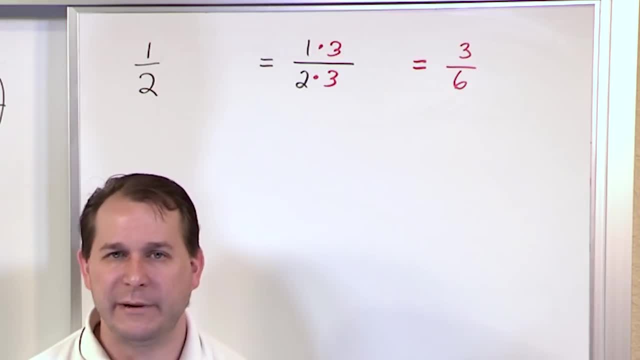 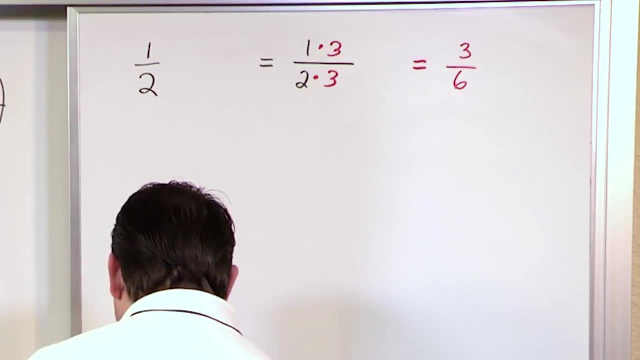 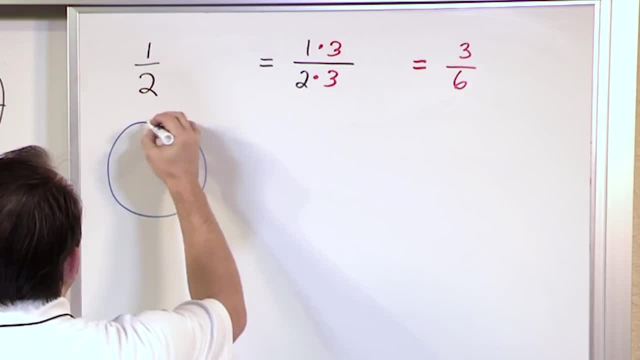 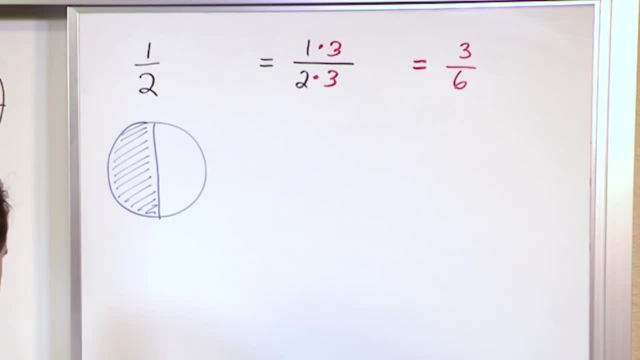 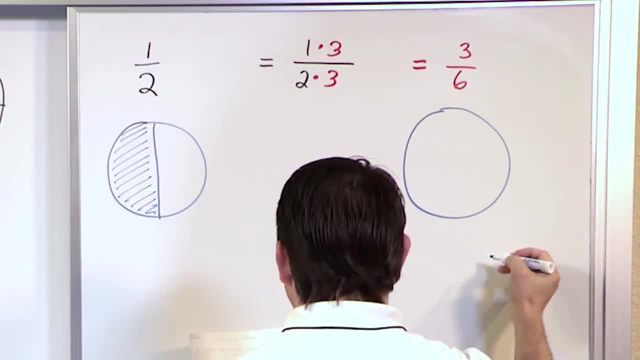 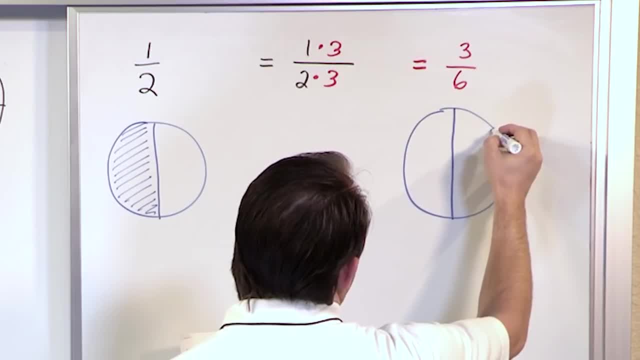 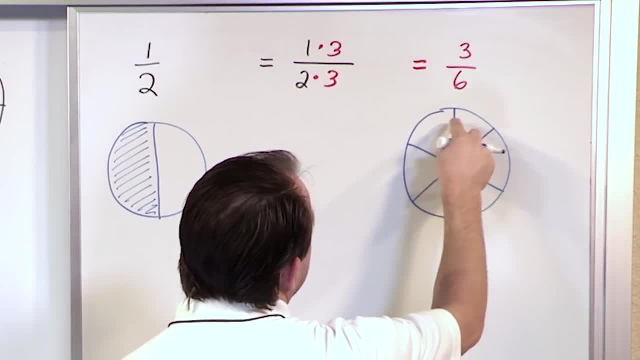 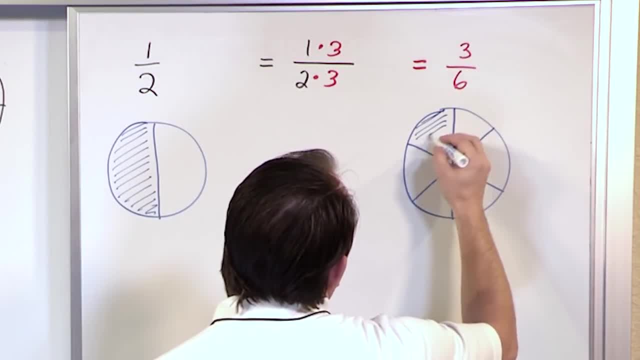 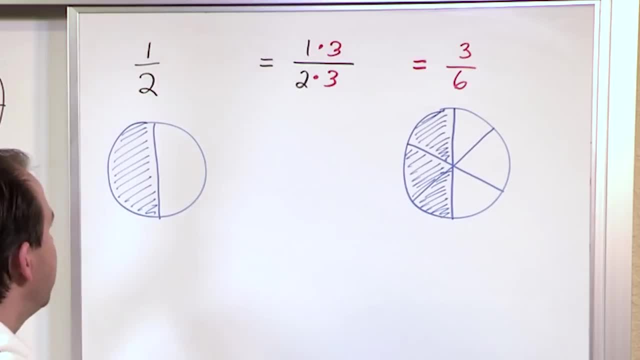 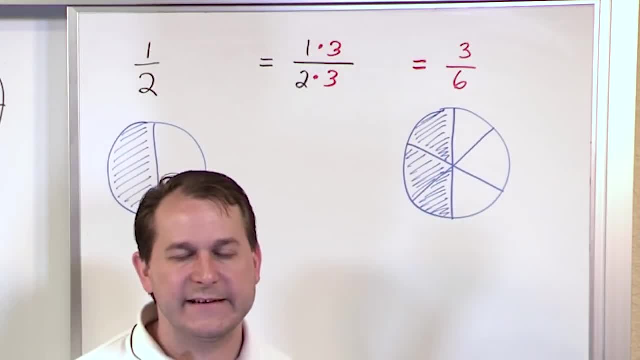 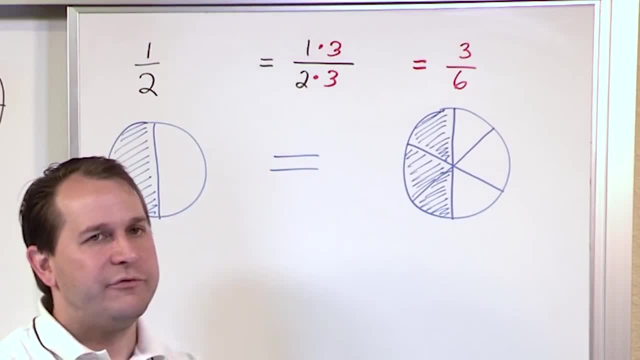 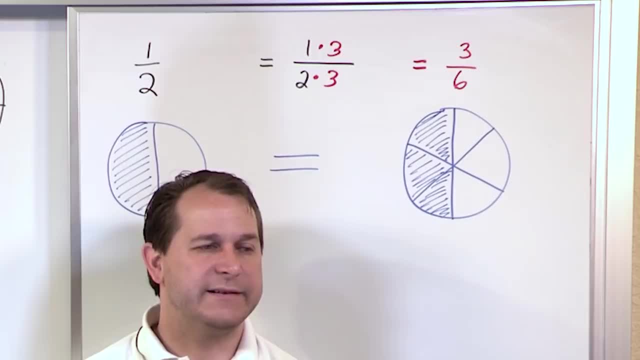 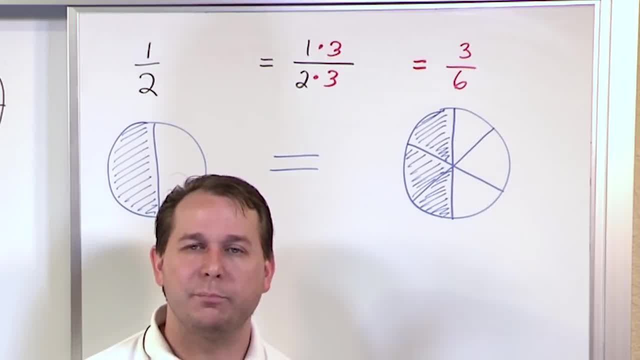 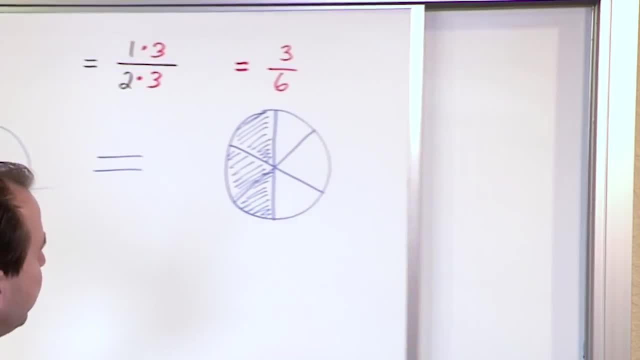 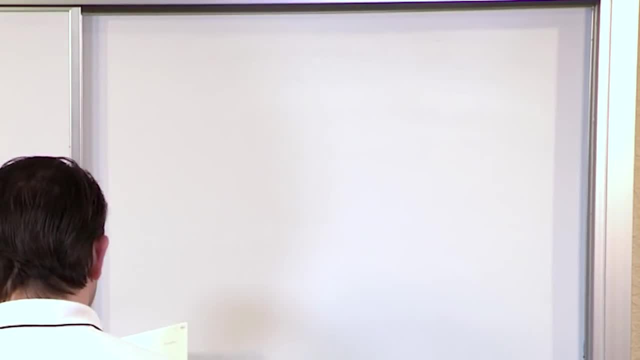 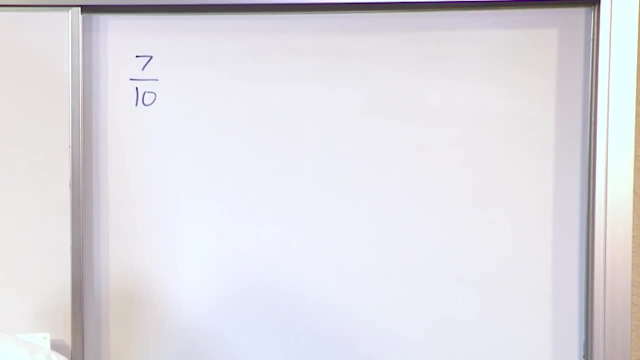 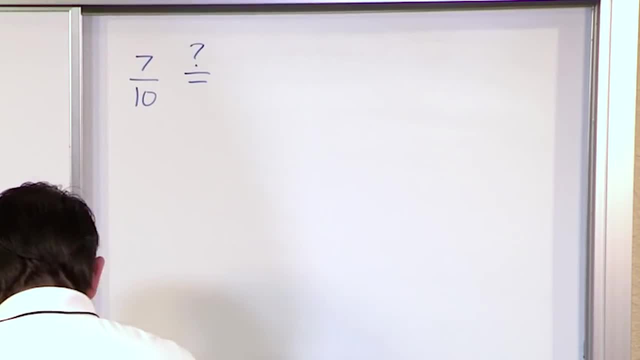 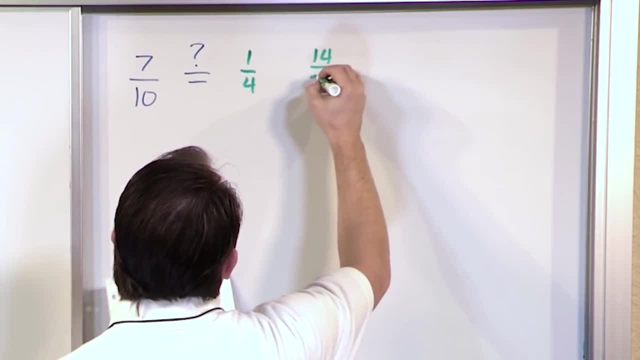 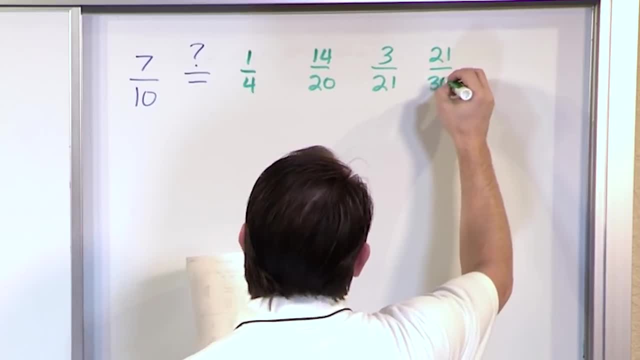 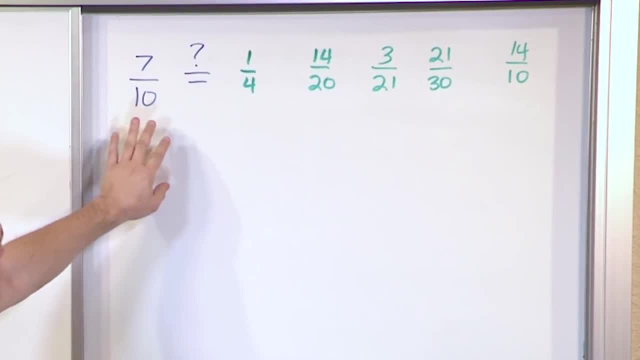 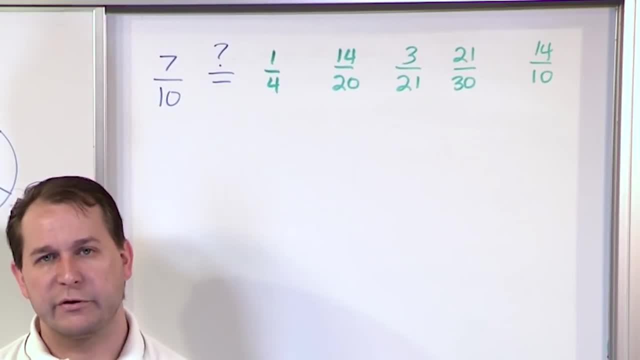 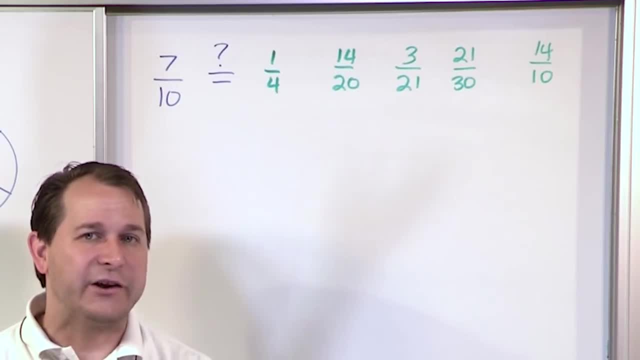 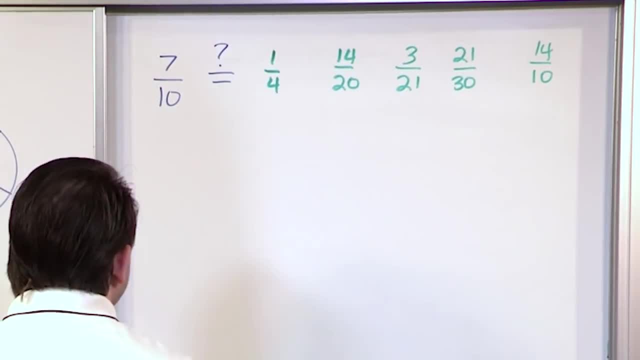 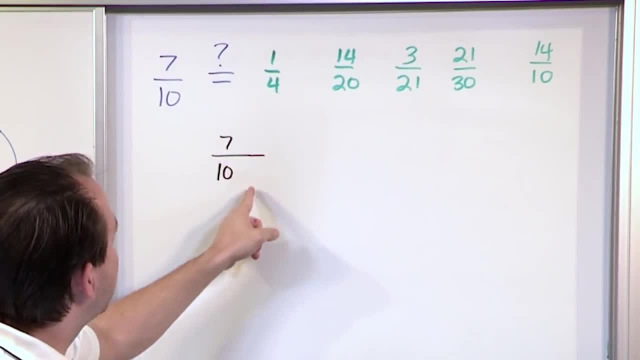 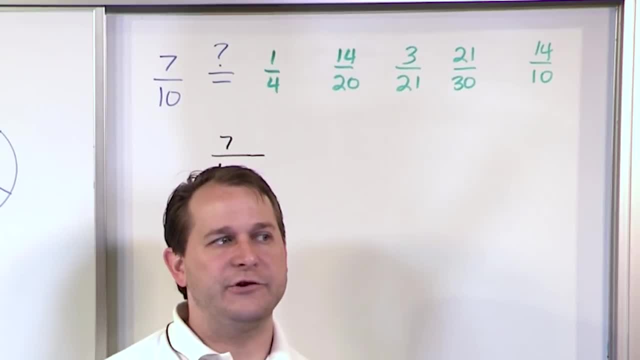 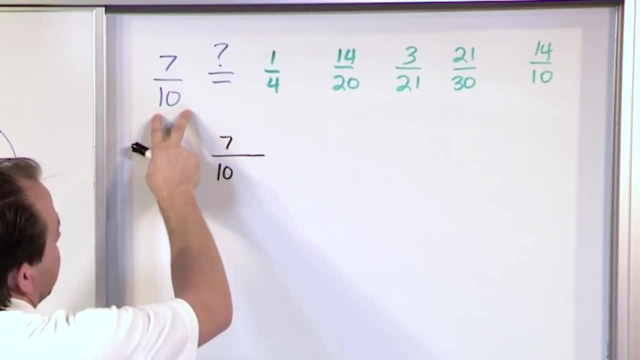 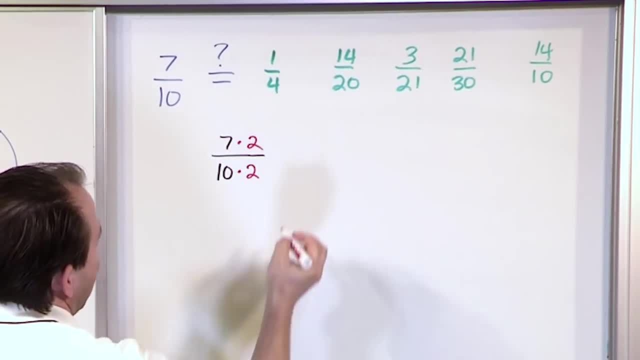 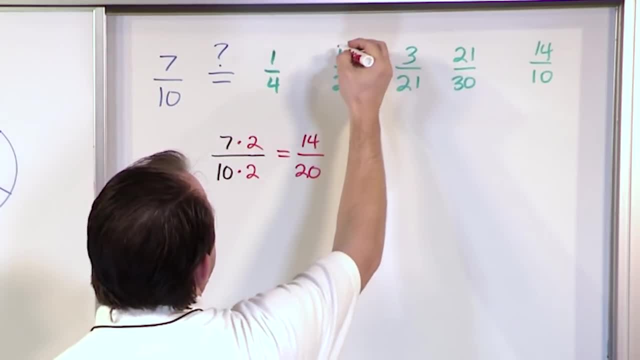 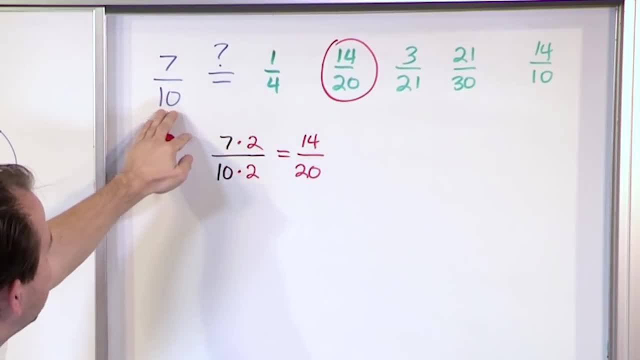 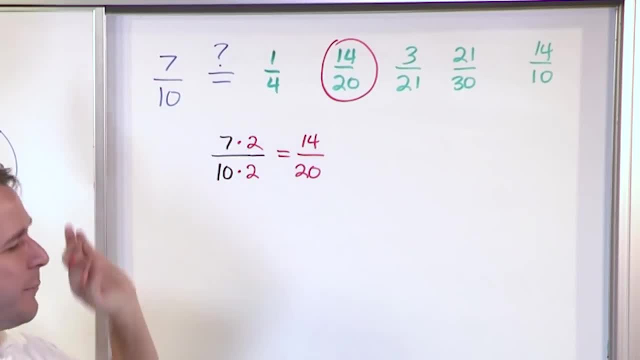 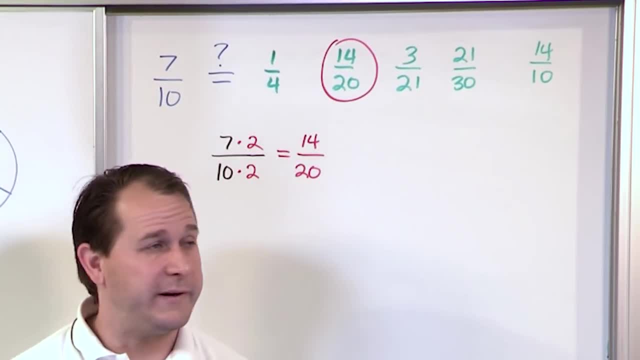 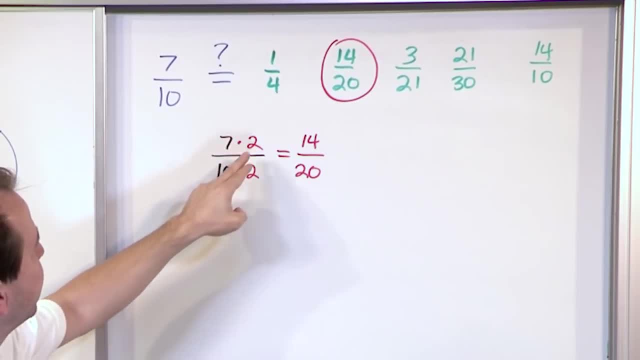 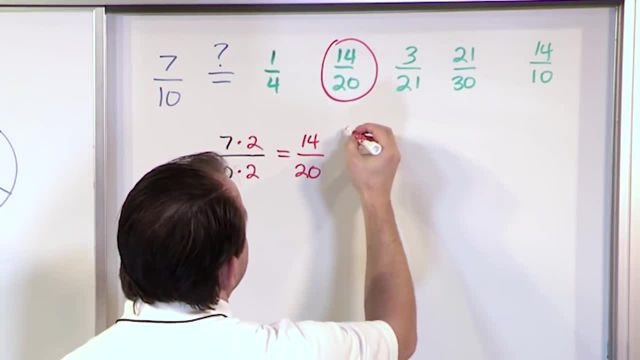 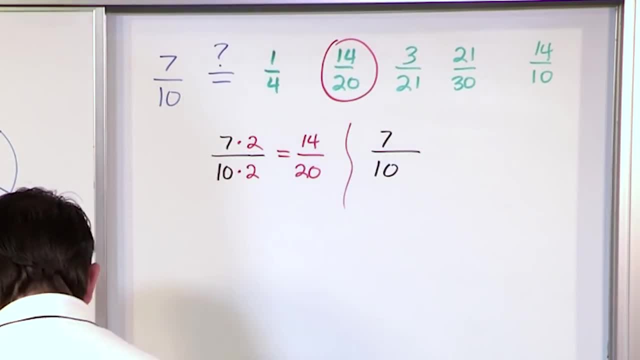 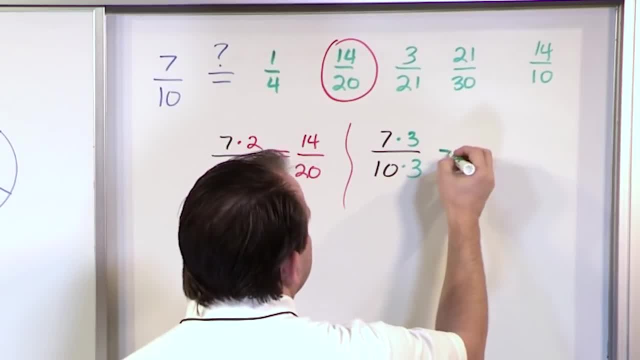 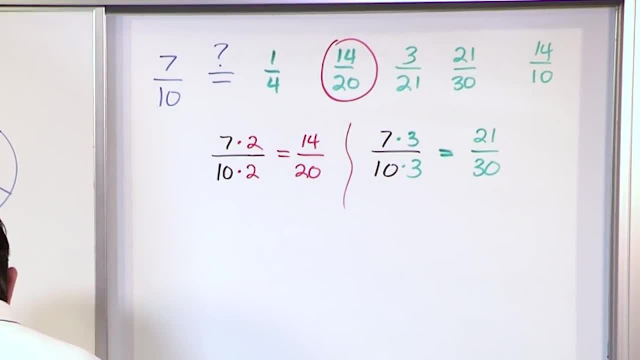 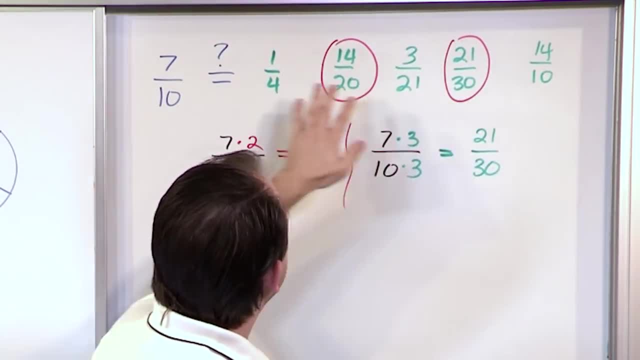 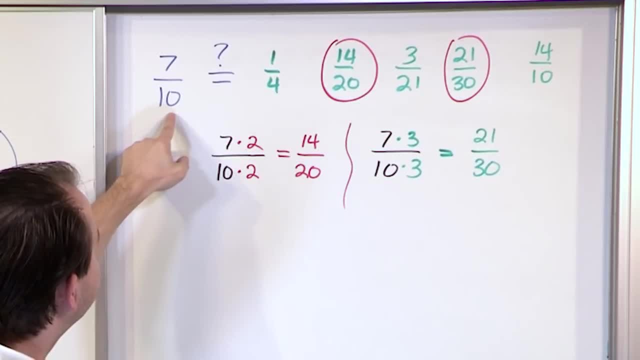 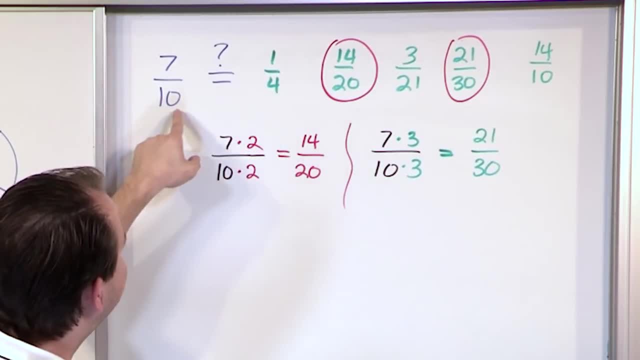 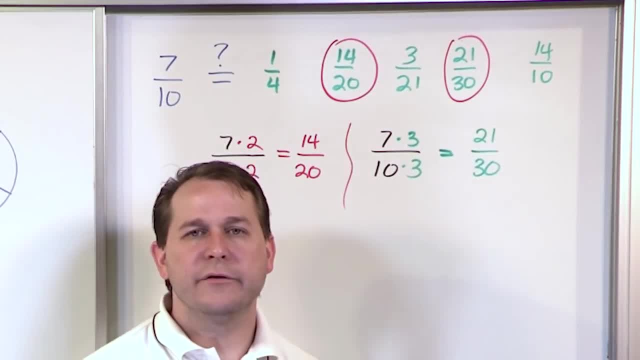 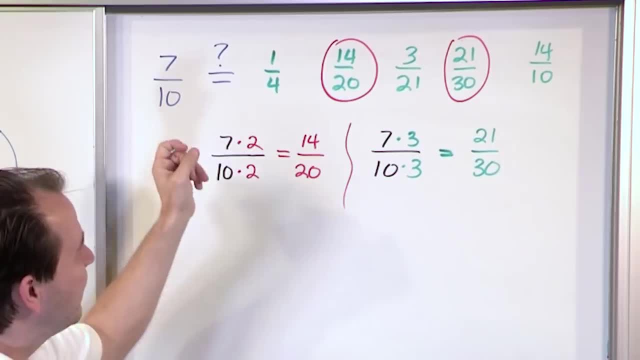 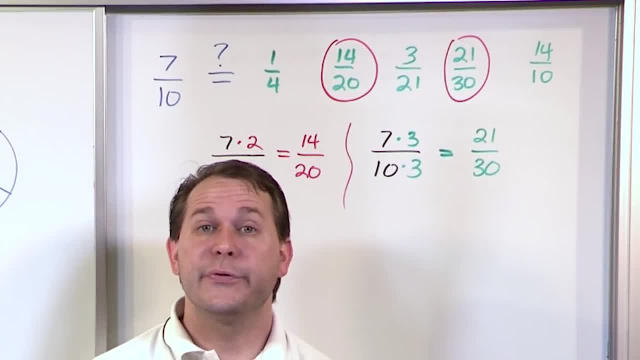 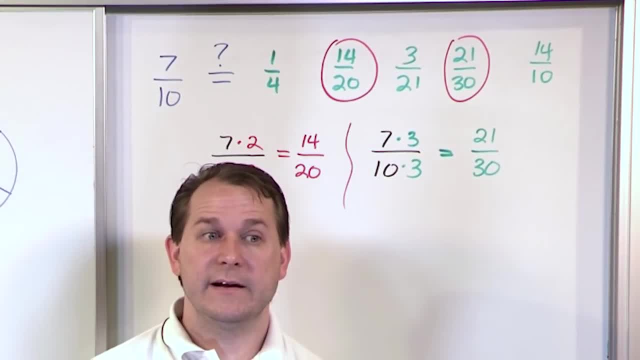 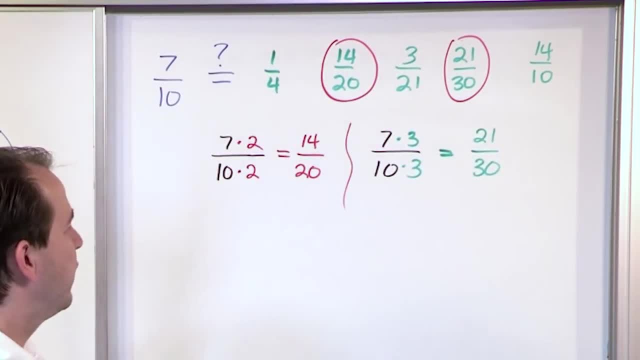 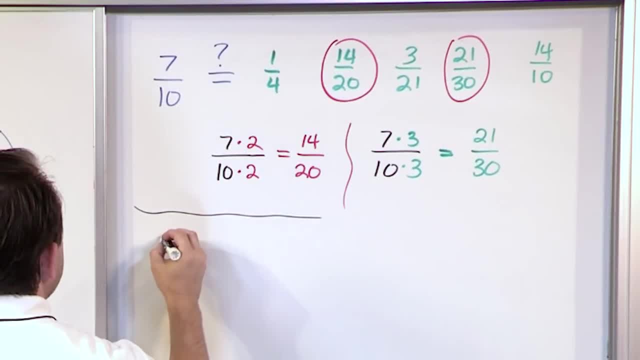 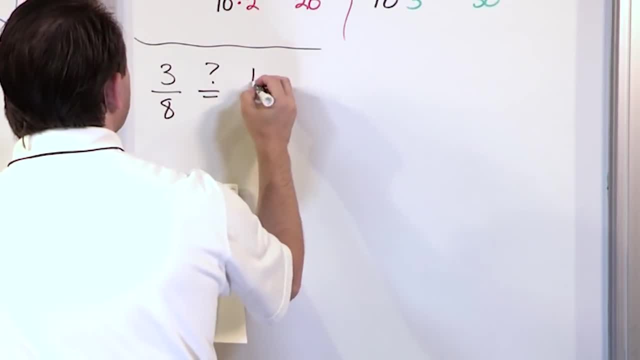 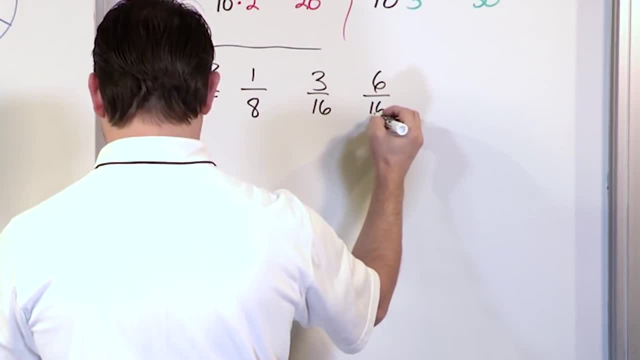 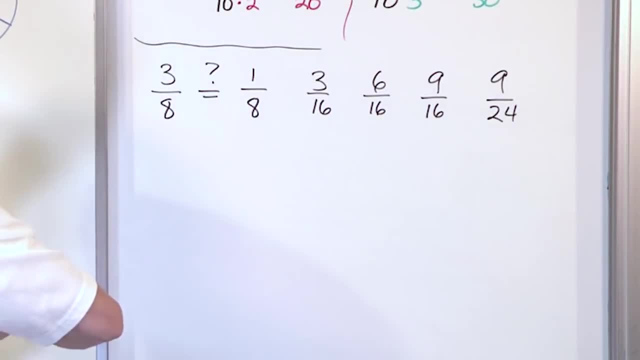 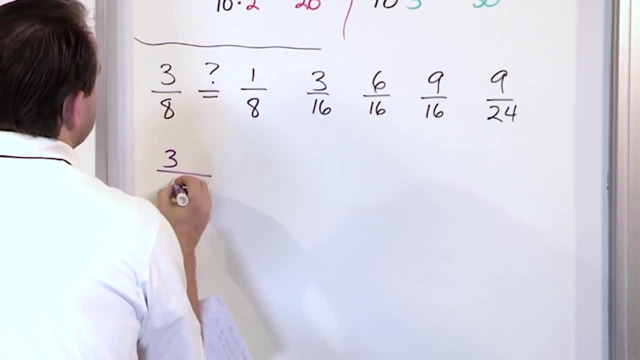 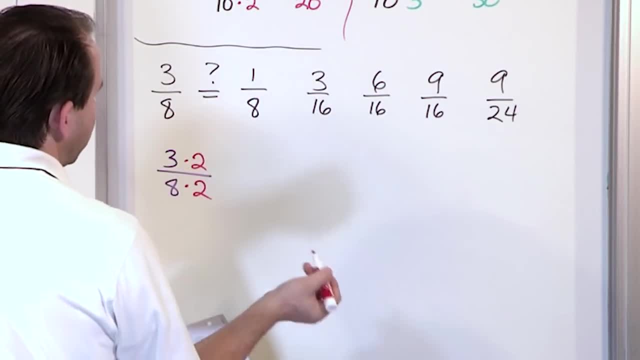 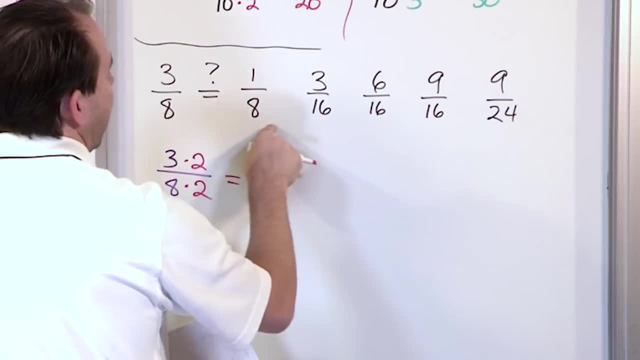 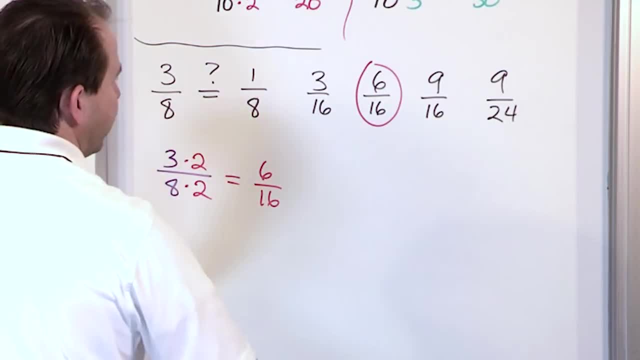 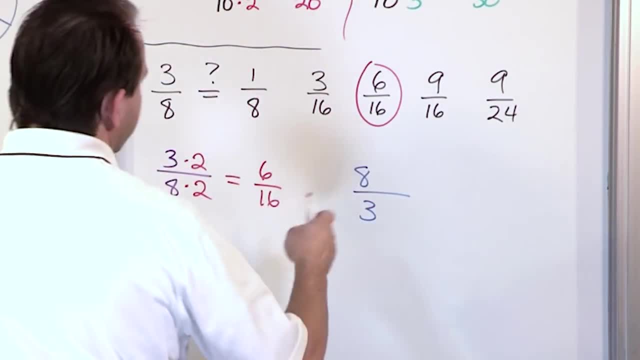 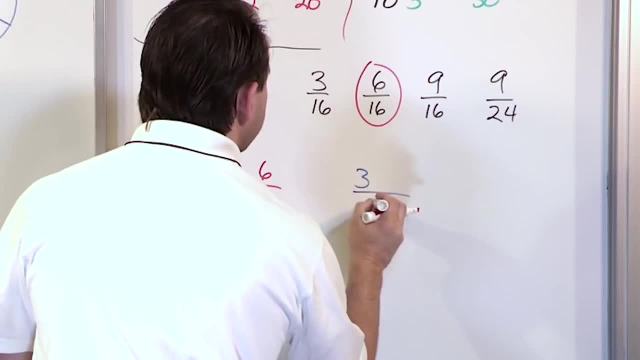 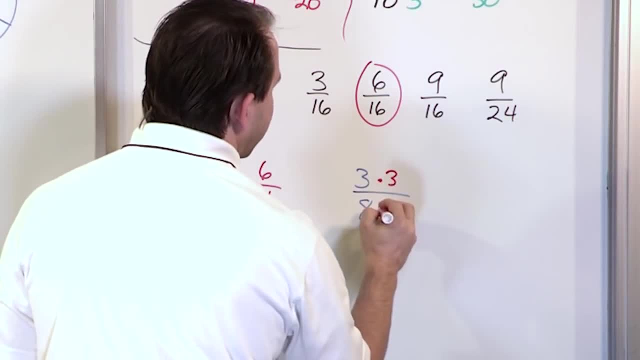 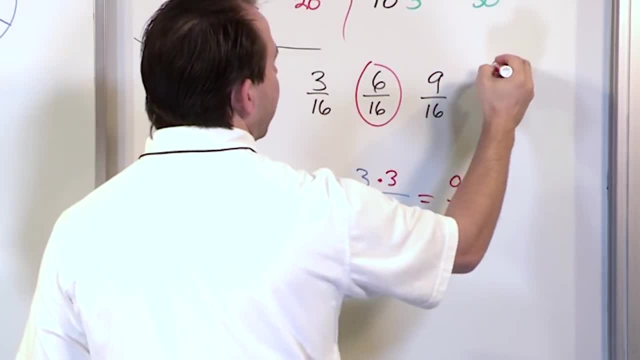 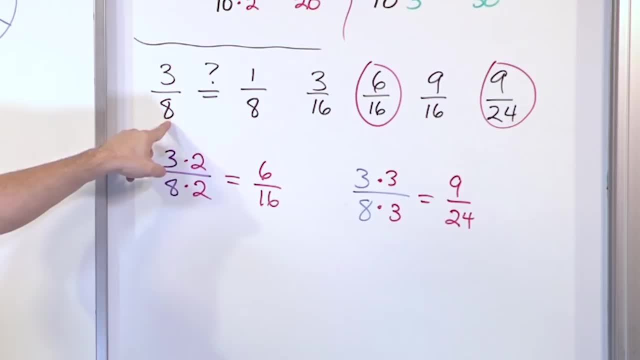 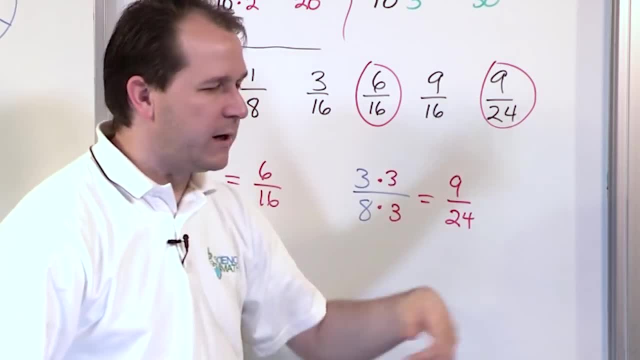 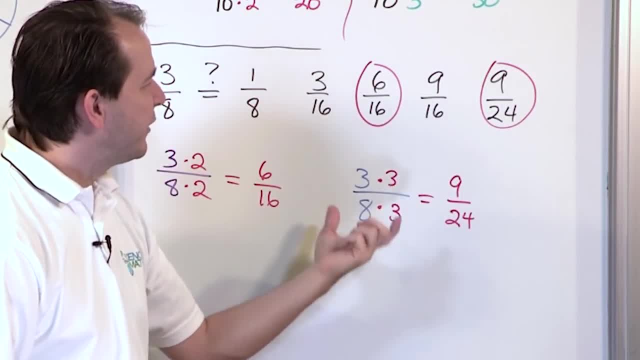 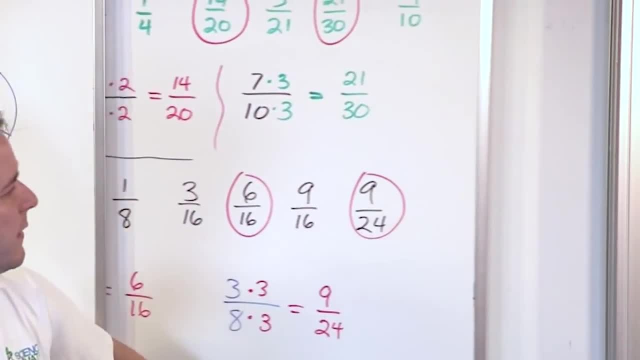 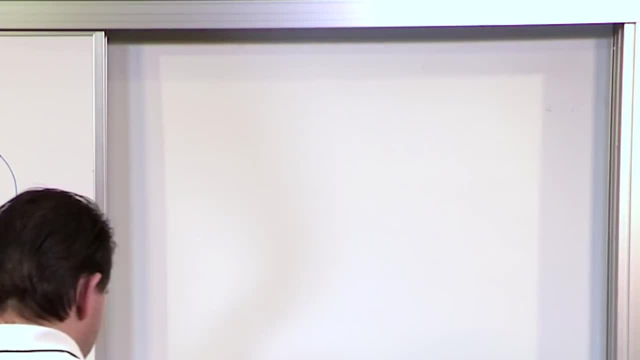 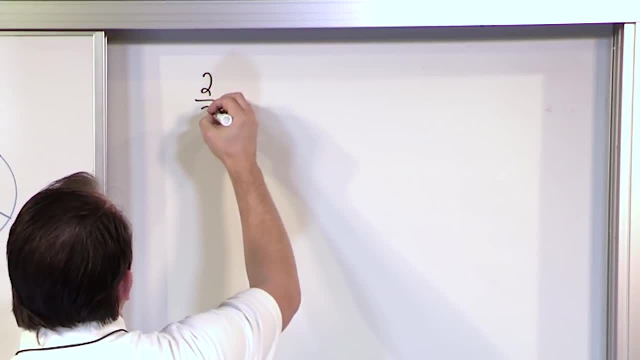 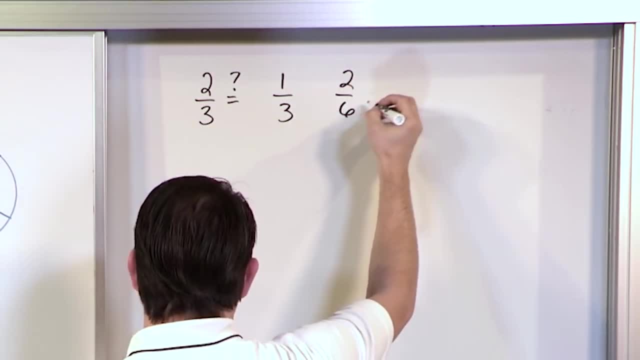 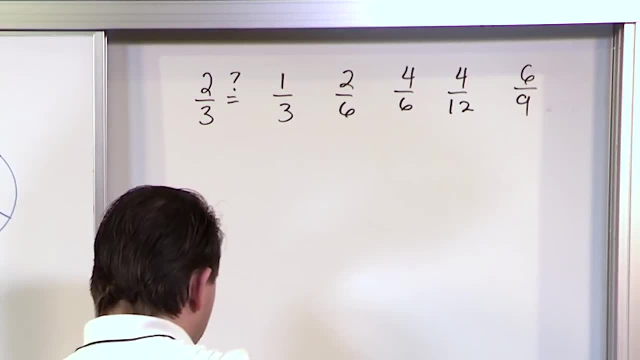 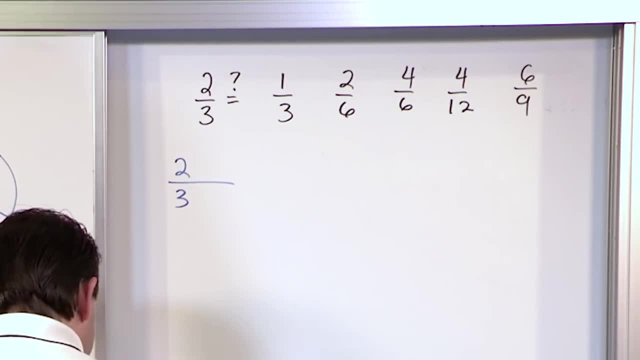 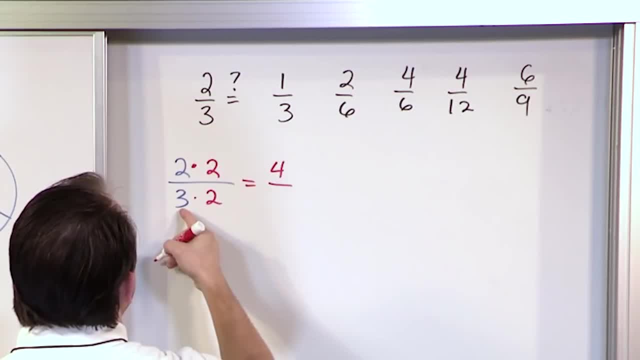 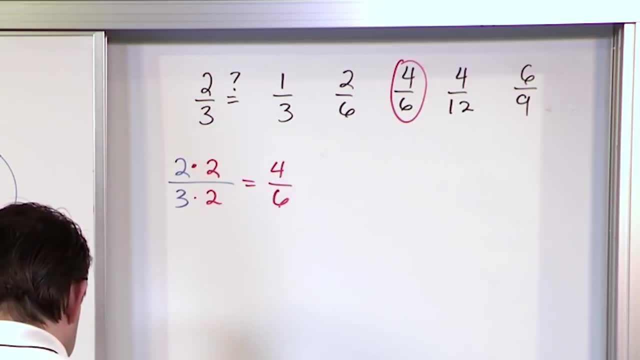 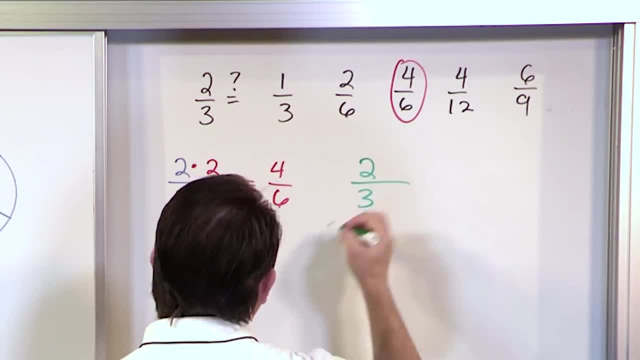 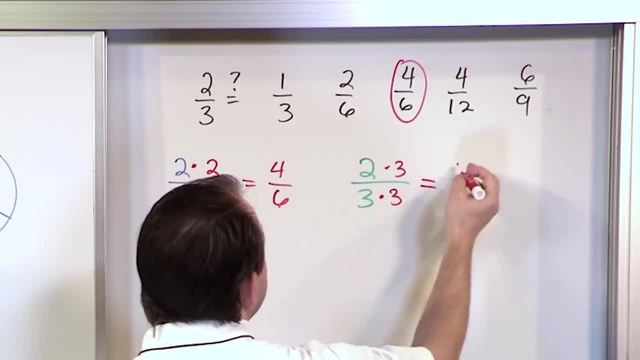 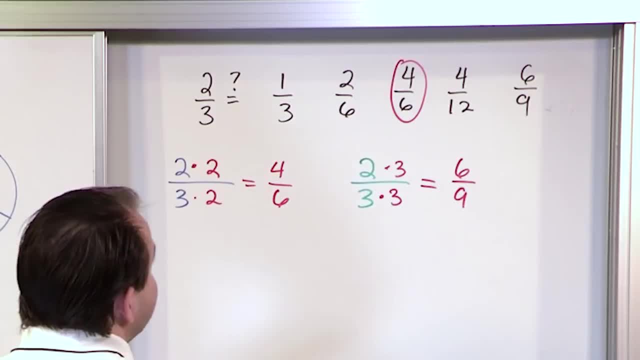 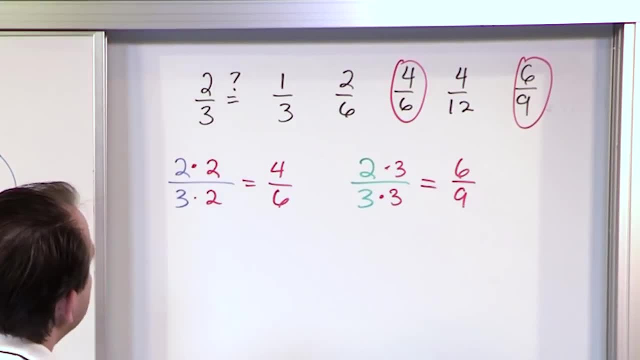 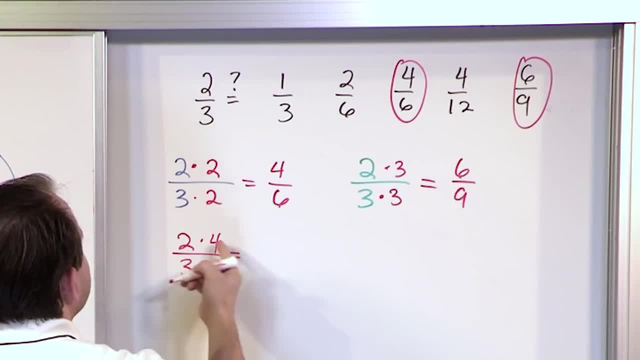 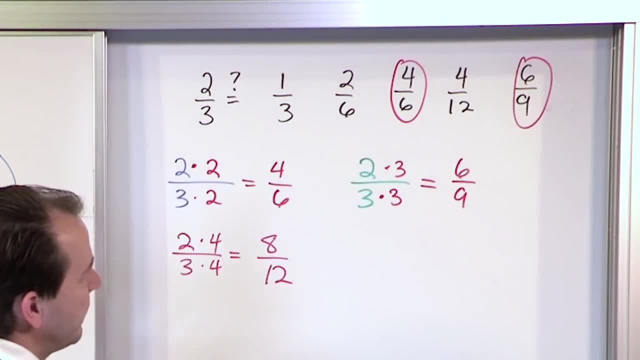 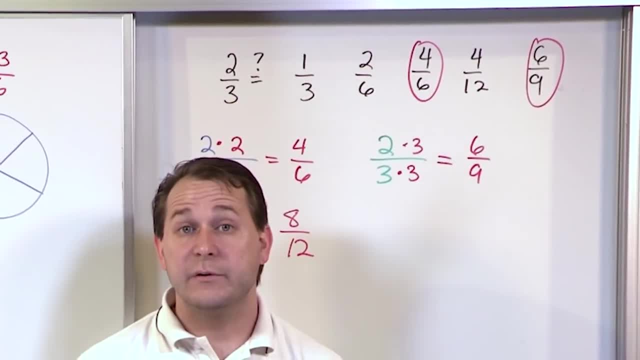 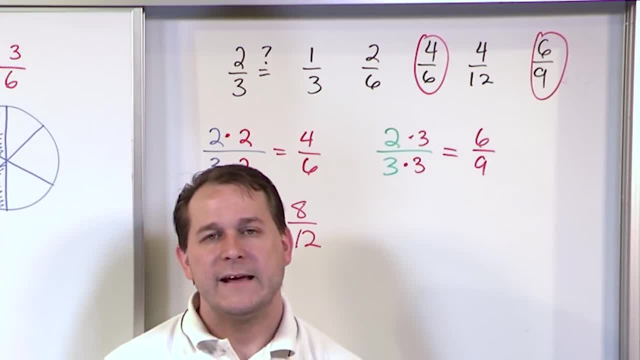 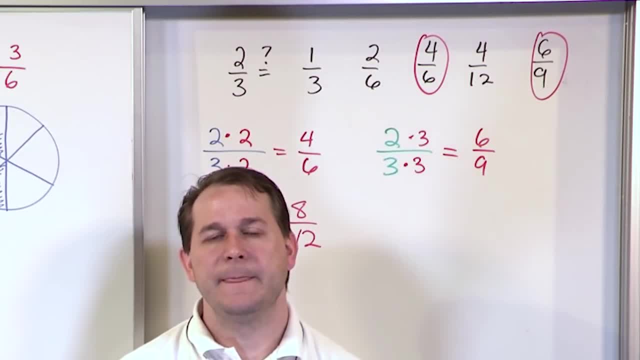 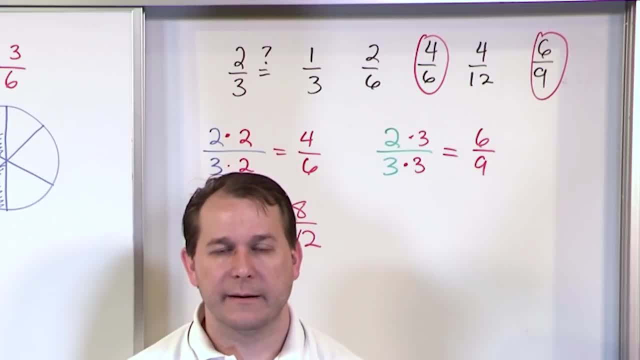 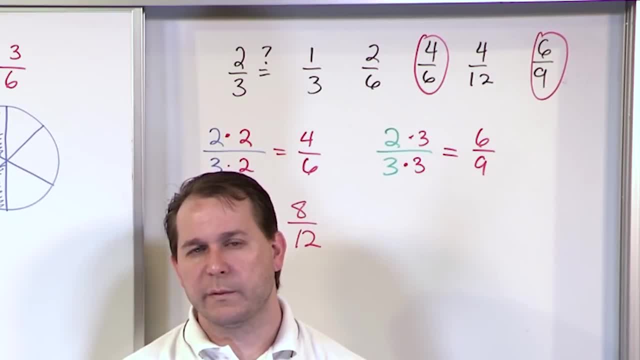 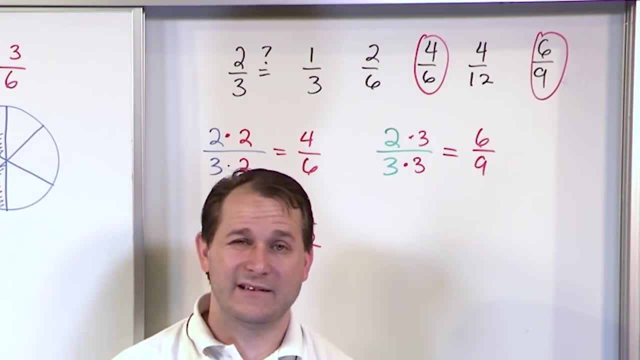 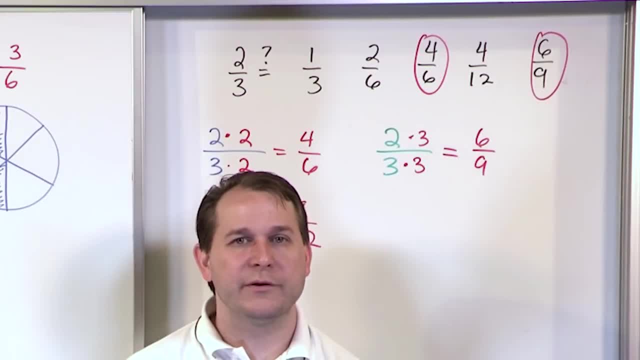 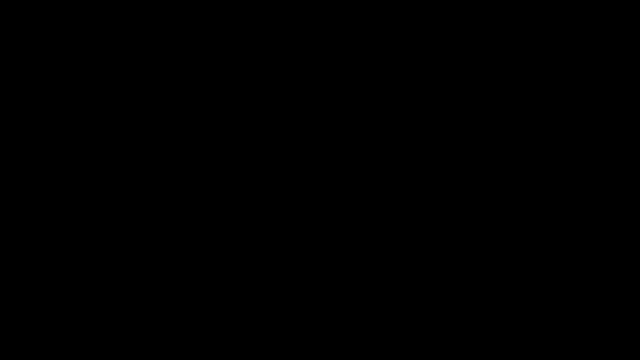 Subtitles by the Amaraorg community. Subtitles by the Amaraorg community. Subtitles by the Amaraorg community. Thank you. 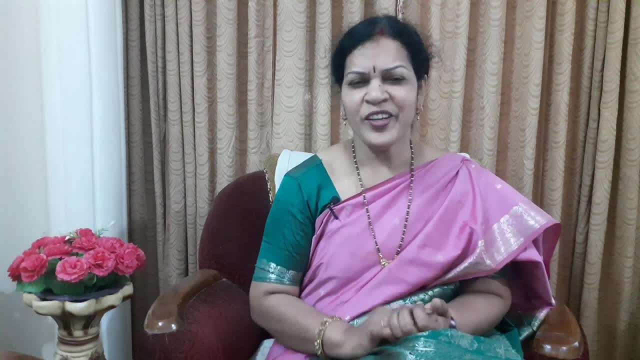 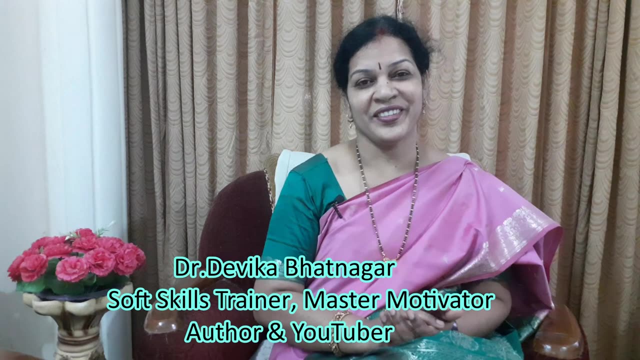 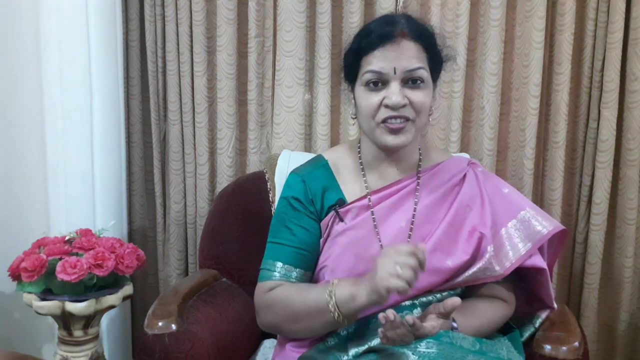 Hello everyone, welcome to Dr Devika Bhatnagar channel. Today I want to give you five golden principles to start teaching field, to enter into teaching field. Five golden principles. This is useful for all the young teachers, young lecturers. 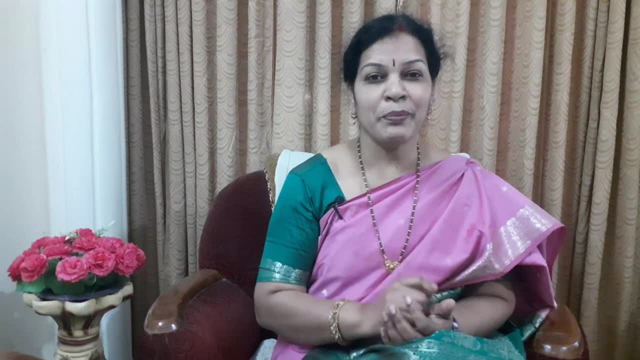 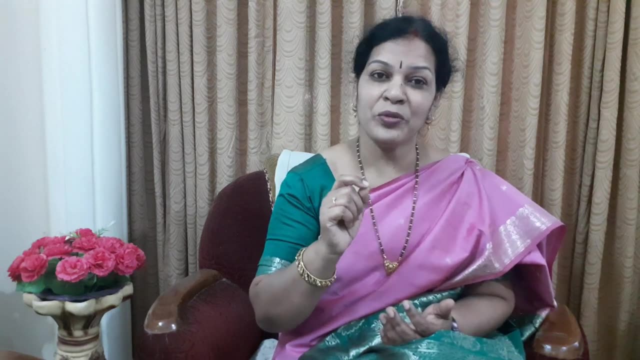 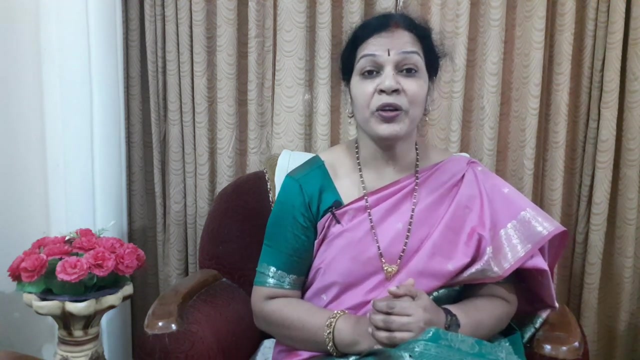 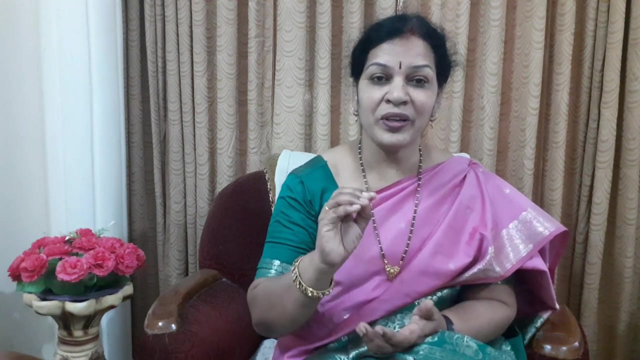 You know that teaching is one of the best profession, Respectable and remarkable, and also one of the best profession. So when you enter into the teaching field, what should be your attitude, What you have to do? This guidance nobody will give you. There is no profession, there is no book is available, But I want to guide you a few things. to all the young faculty: